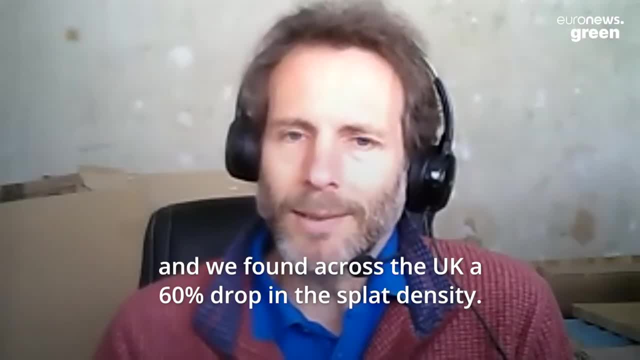 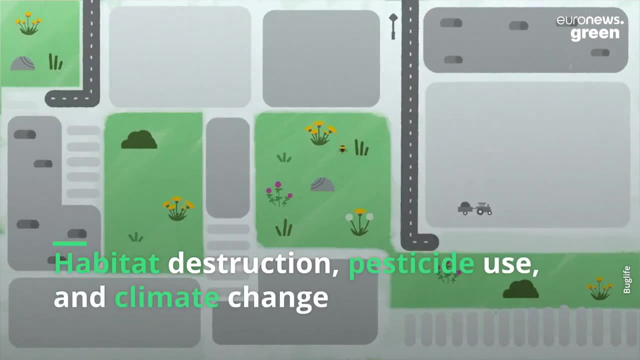 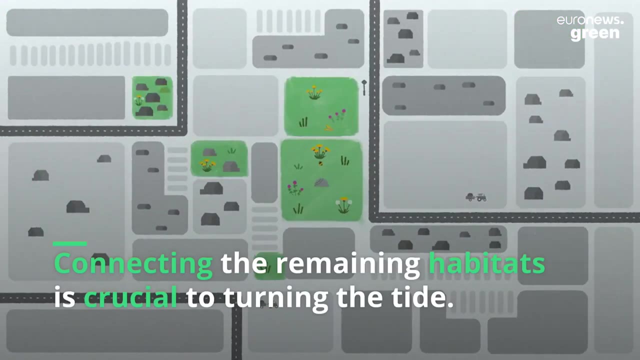 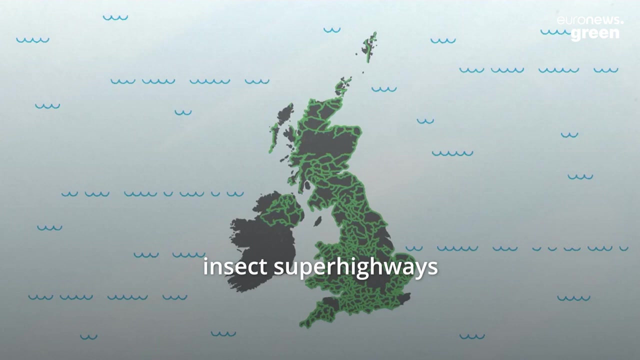 out and we have found across the UK a 60% drop in the splat density. In the UK we've developed the Bee Lines Network of Insect Superhighways or the concept of the wildlife corridor. It's very, very important. 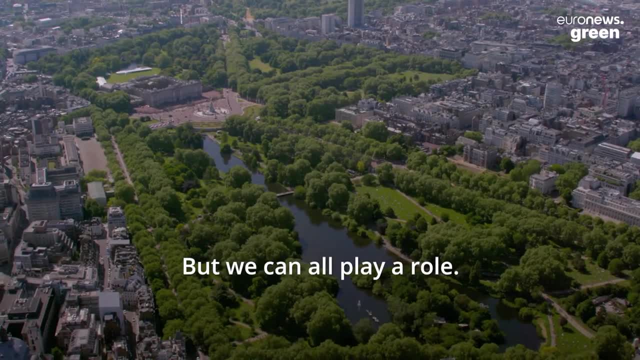 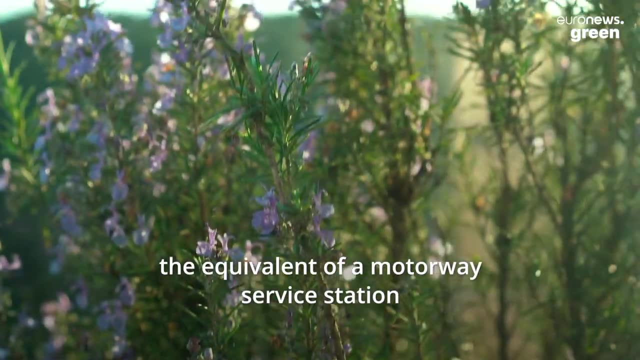 that we bring these connectivity back in. But we can all play a role If nothing else. for instance, if you planted a group of herbs and you let them flower, you've created the equivalent of a motorway service station where pollinators can drop off fill themselves. 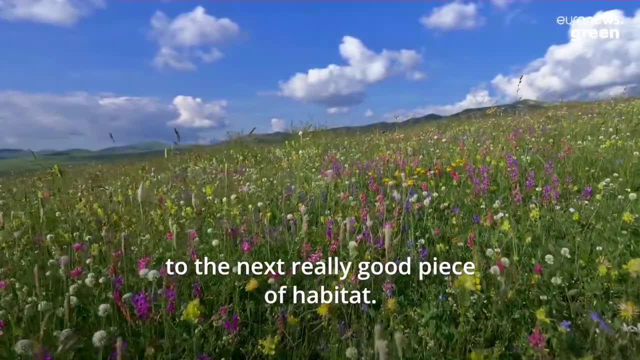 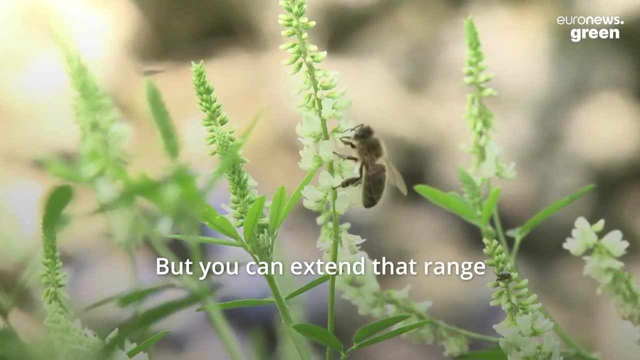 up and be able to make the distance to the next really good piece of habitat, Because a lot of our pollinators can only travel 300, 400 odd metres, So they haven't got a large range. but you can extend that range by putting some good plants in the right. place. 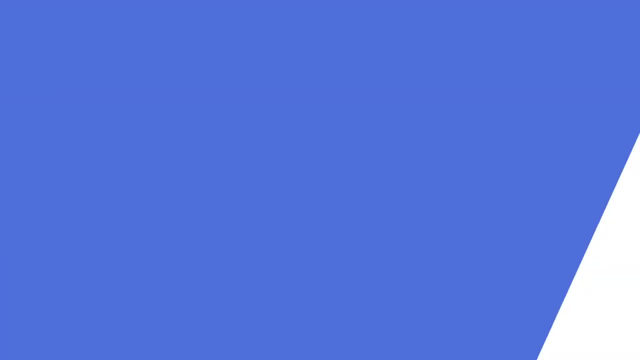 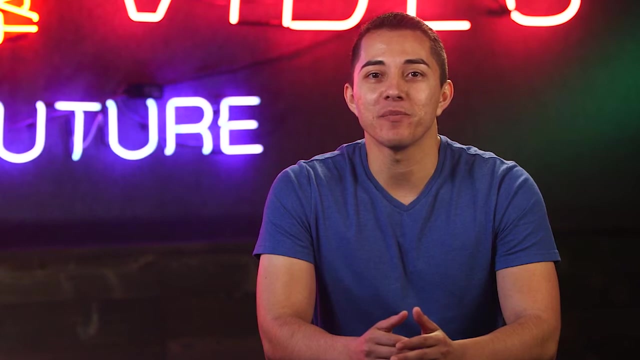 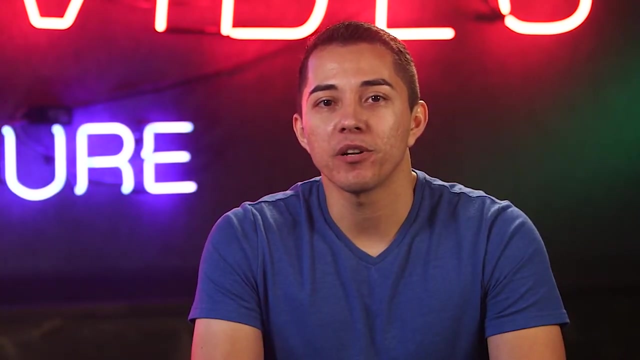 Computers are able to communicate across massive distances at near instant speeds. It's a remarkable technical advancement at the root of how billions of people use the Internet every single day. Earlier in this course, we learned about how computers communicate with each other over short distances or on a single network segment or LAN. 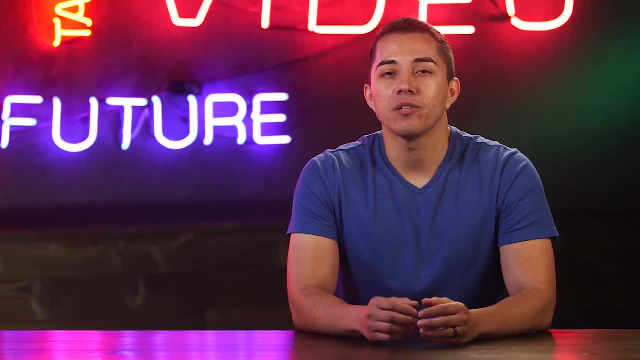 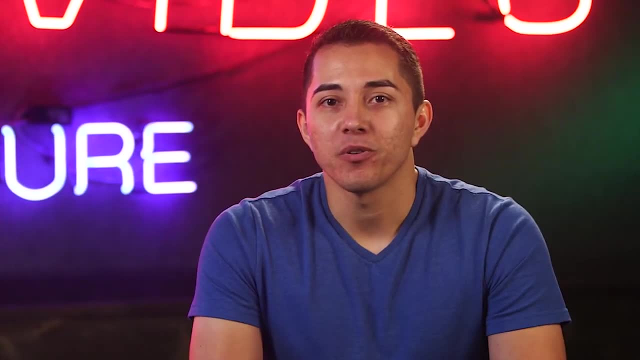 In these next lessons, we'll focus on the technologies that allow data to cross many networks, facilitating communications over great distances. By the end of this module, you'll be able to describe the IP addressing scheme and how subnetting works. This means you'll learn how to perform basic math in binary in order to describe subnets. 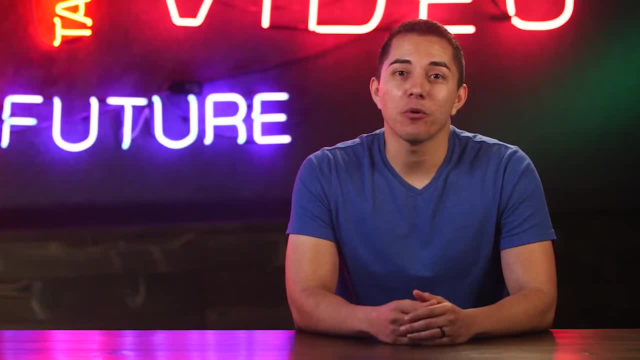 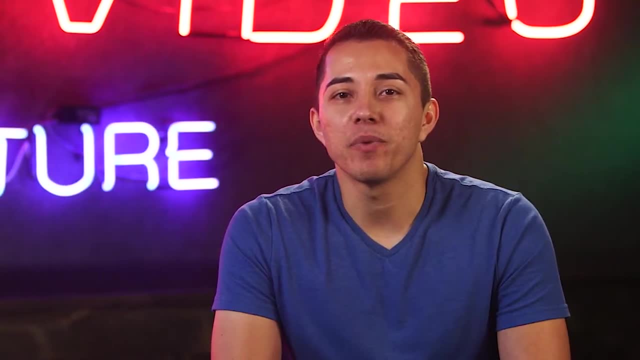 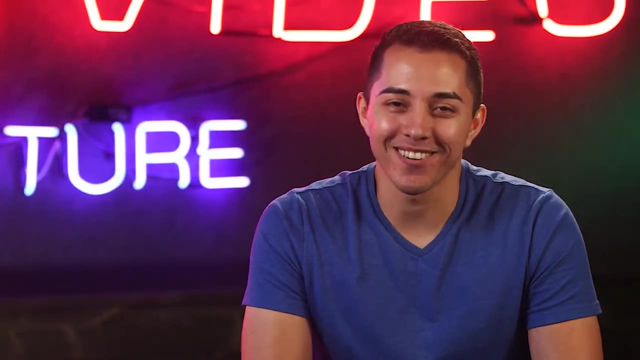 You'll also be able to demonstrate how encapsulation works and how protocols such as ARP allow different layers of the network to communicate. And finally, you'll gain an understanding of the basics behind routing, routing protocols and how the Internet works. For now, route yourself to the next video and we'll get started. 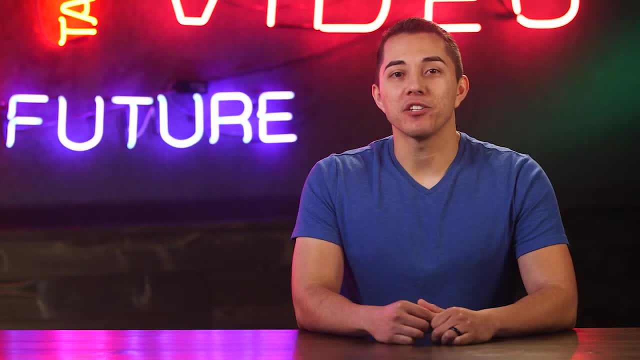 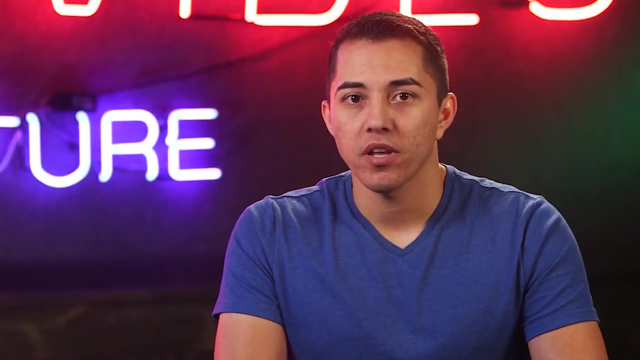 On a local area network or LAN nodes can communicate with each other through their physical MAC addresses. This works well on small scale because switches can quickly learn the MAC addresses connected to each of their ports to forward transmissions appropriately. But MAC addressing isn't a scheme that scales well.